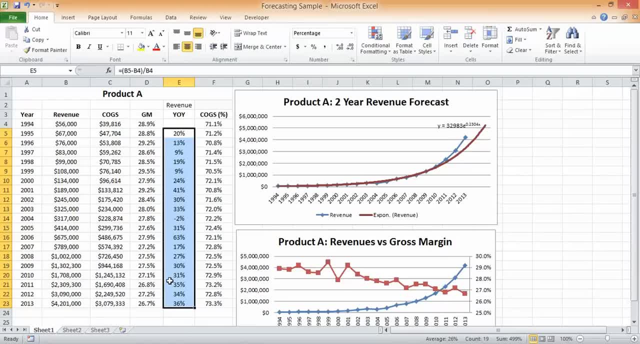 tricks on how you can make this kind of a chart look really nice visually. If you don't know how I calculated these year-over-year revenue increases or decreases or are interested in learning on how to do that, I did post a video earlier on how to create these calculations in. 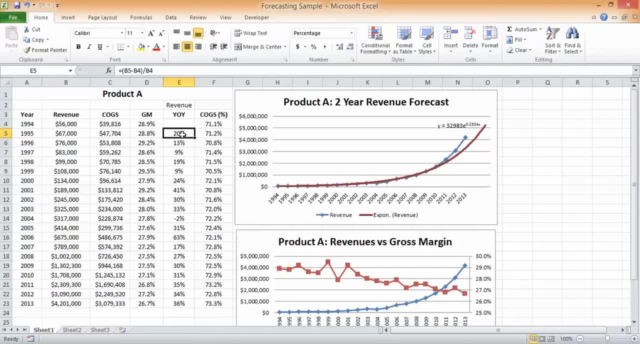 here for each year. so you'll want to take a look at that. What I'm going to start out with in creating this chart is selecting cells E5 through E23. That's the entire series here of these increases or decreases percentage. I'm going to use a column, graph 2D column. make it pretty easy to display this. Make. 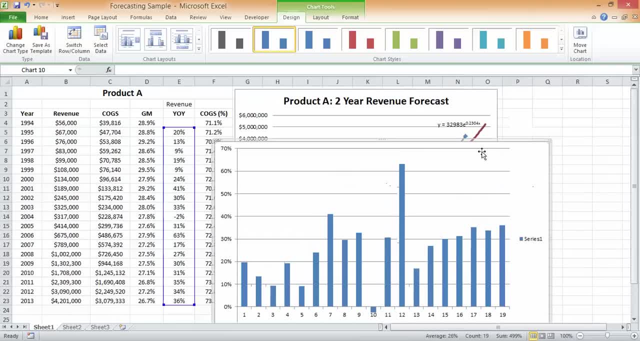 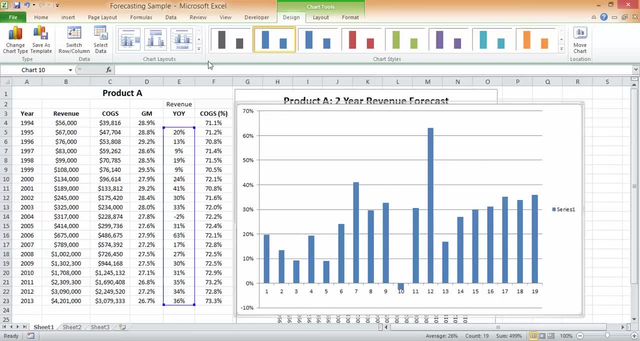 this bigger so you can see this while we're working on it, And what I'm going to do is go back up to layout Again, you can always select whatever layout you want to work with for whatever kind of chart it is you're creating. I like to use layout three, so I'm going to select that. I'm going to clean this up. 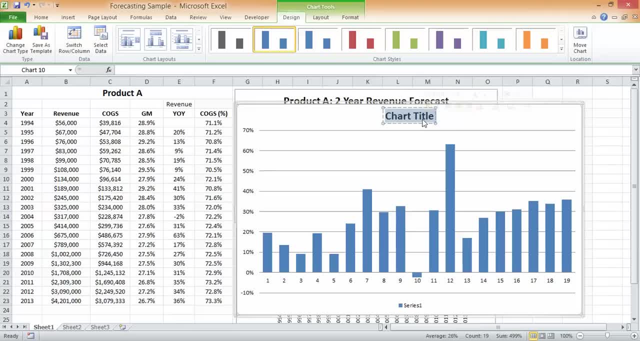 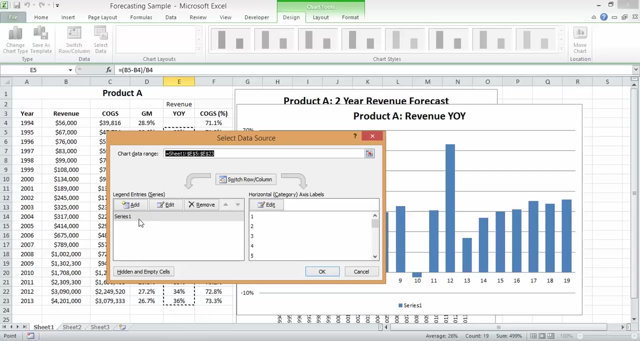 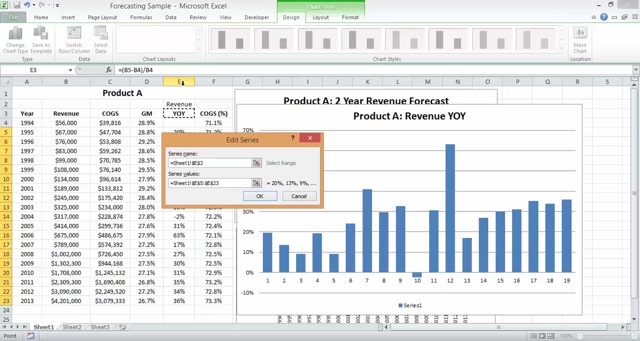 a little bit here. I'm going to call this product A revenue year-over-year Okay. And another thing I'm going to do to clean this up a little bit is go to the select data And I'm going to rename this series, one which is really just our year-over-year percentages, as year-over-year, which is the. 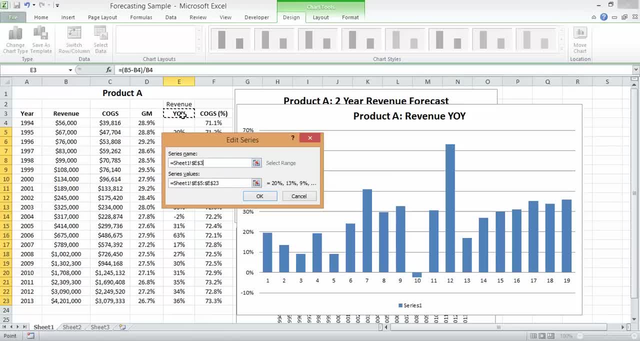 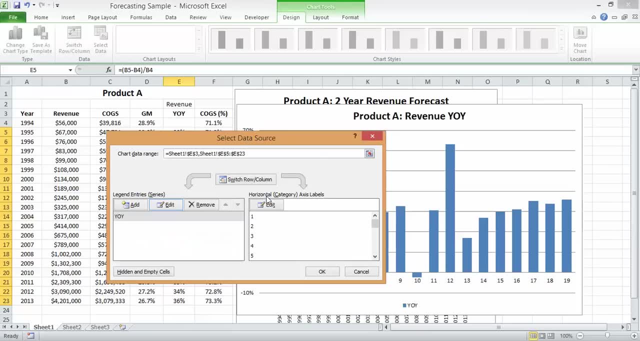 contents of cell E3.. You could also just type in as free text whatever you want to call it in this series name right here and click okay. You can see that changed this from series one to year-over-year. Next I'm going to change these horizontal axes. As you can see, I have to use a Lock. look at the. 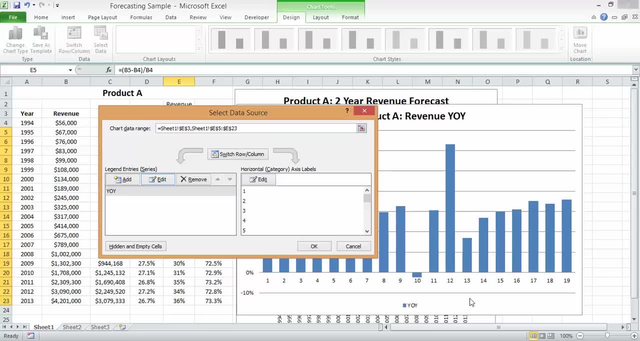 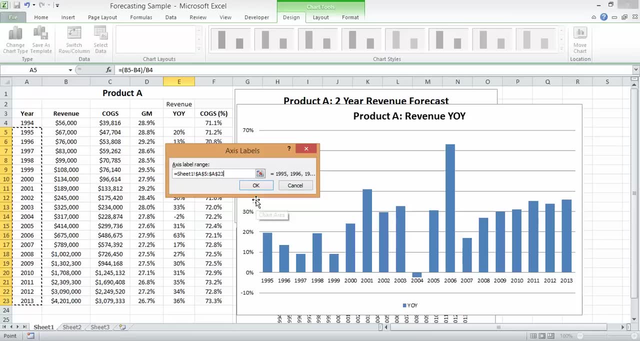 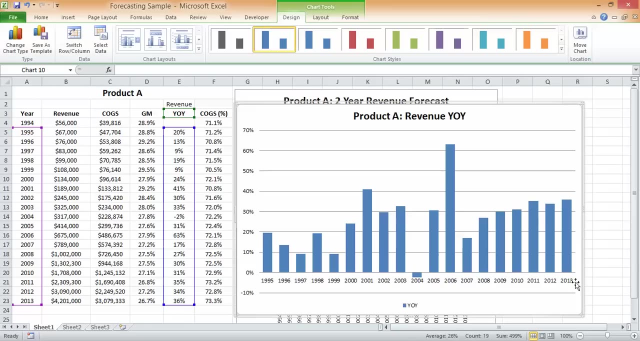 labels from how they're currently appearing: 1 through 19 to 95 through 2013. click OK, click OK again and you can see now that changed to 95 through 2013, so it appears a little cleaner. going to next go up to these chart styles and I'm 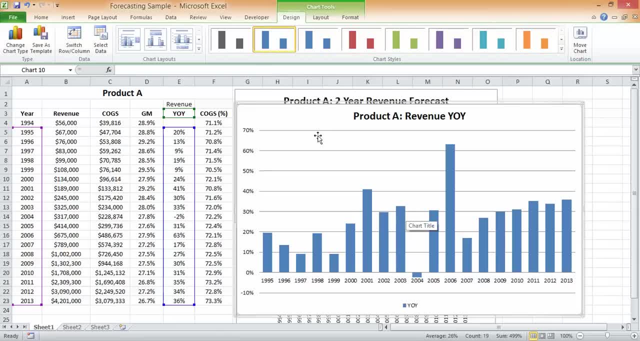 going to change these, the fills of each of these bars, from blue to green- and in my mind, that's gonna any. any green bar is gonna represent a positive year-over-year increase. now, we did have this one year, in 2014, where there was a year-over-year. 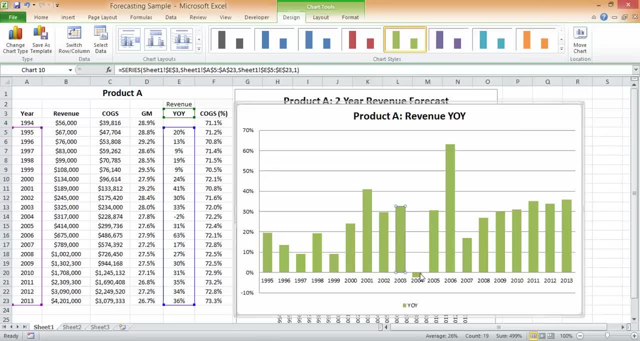 decrease, and what I'm going to do is just click on that bar. okay, you notice, when I first clicked on one of the bars here, it selected all of them, and then when I click a second time on the individual bar, it just selects that one bar. so I've got just this one bar selected and all I'm going to do is. 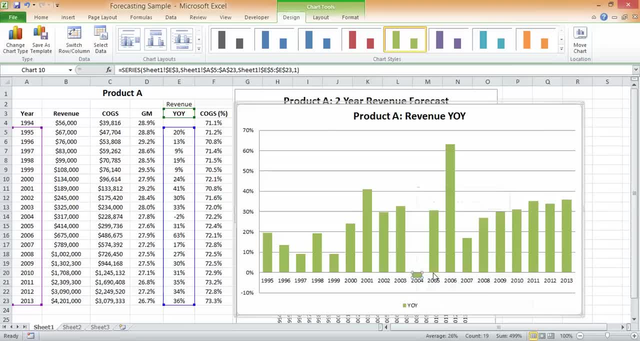 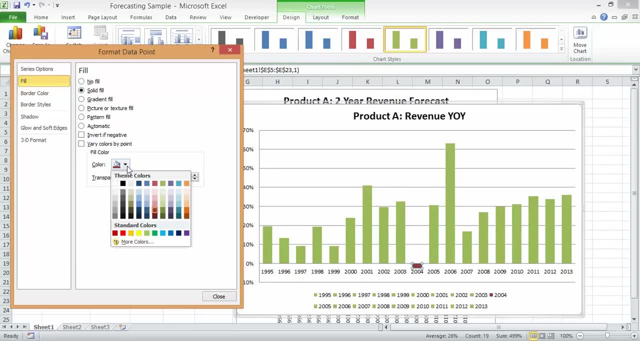 right-click on it and I'm going to click on format data point and I'm gonna go over here to fill and I'm gonna go to solid fill and I'm going to select this red color. actually, I'm going to go back and select that darker shade of red in. 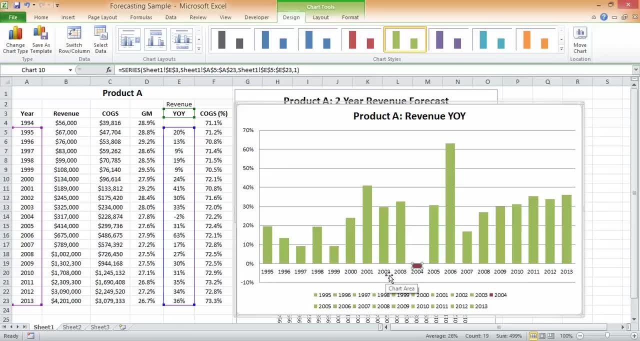 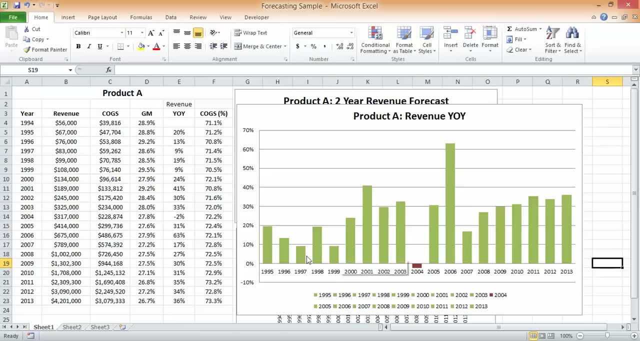 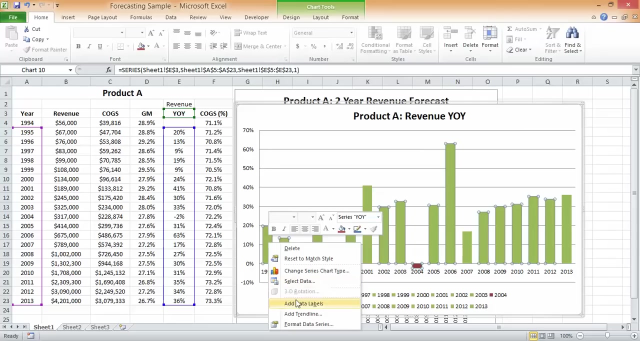 there and I'm going to click close. and now you can see that we have green bars for all of the positive growth years and then one red bar for that year that we had a decrease year-over-year. now another thing I can do is add in what's called 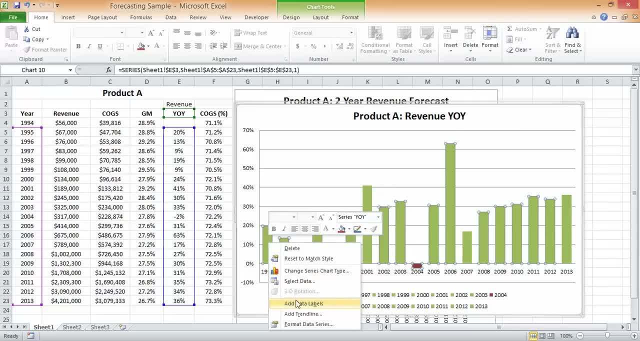 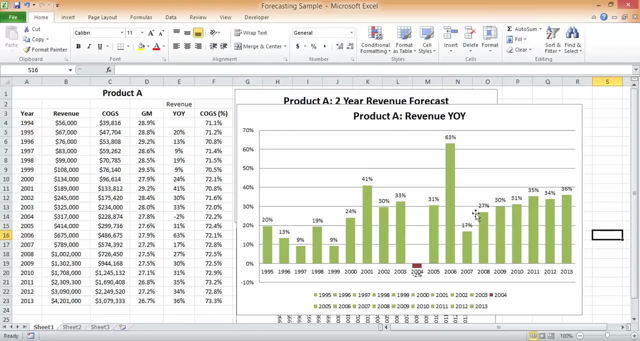 data labels to this chart and what that's going to do is display now each of these percentages is year-over-year increases or decreases- right on to the chart itself. so it calls them right out on there and we can see what the growth percentages was were for each given year. now this negative 2% is: 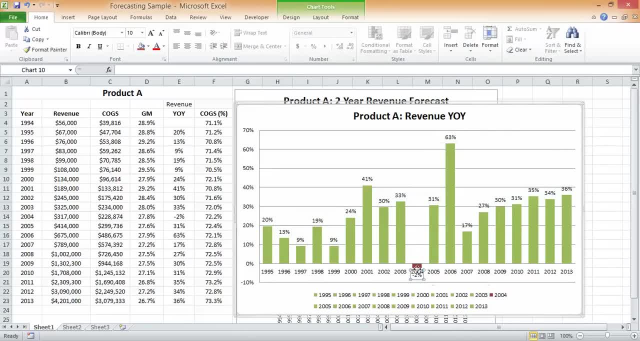 kind of stuck down here, and so I'm going to just pull it up so that we can make sure it's visible on the graph, and that just demonstrates how you can move these around. you can see that we've got a lot of growth here and we've got a lot of. 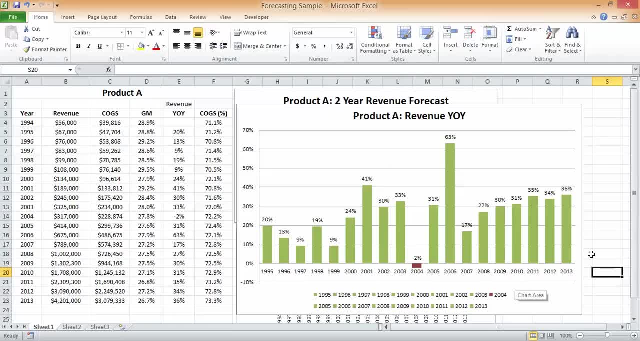 growth right here as well, so we can see that we've got a lot of growth here, and then we can just move these data labels around a little bit if you need to for any of the data points. okay, so we have a nice little chart here showing all of